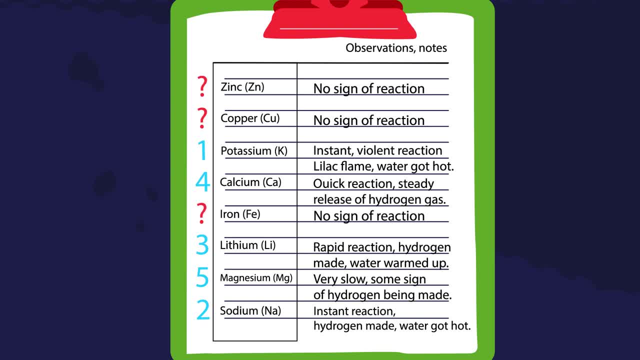 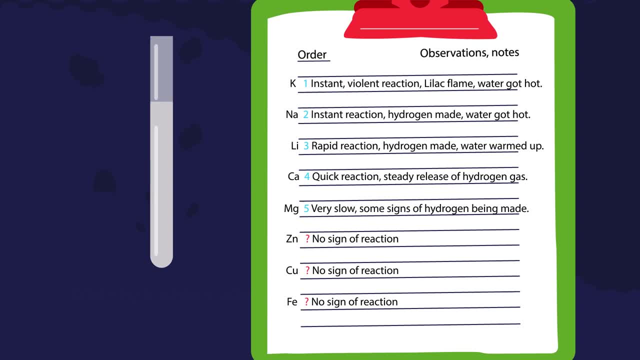 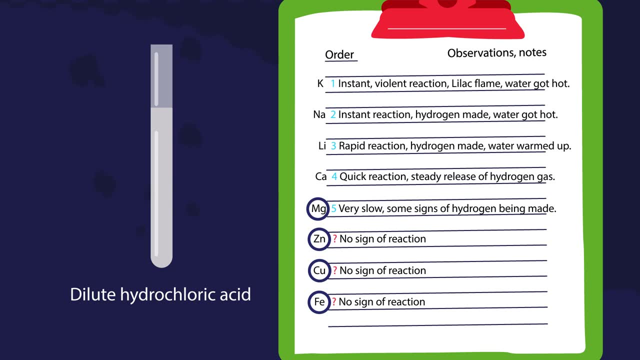 From the results, some can be ranked, but others appear to be the same. Let's rewrite the list. If the experiment is repeated with dilute hydrochloric acid, we can reveal the different chemical reactivity of the metals that have not yet been ranked. 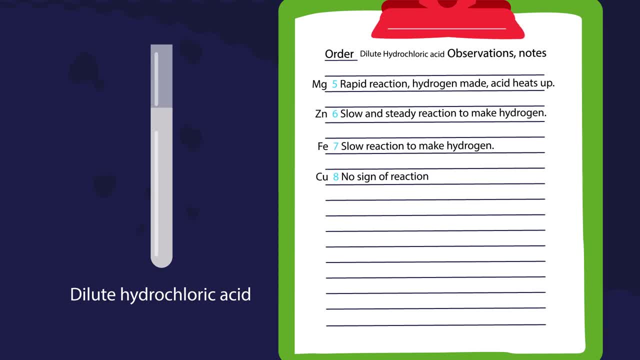 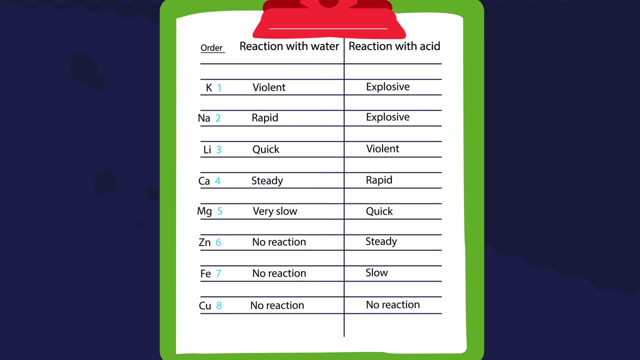 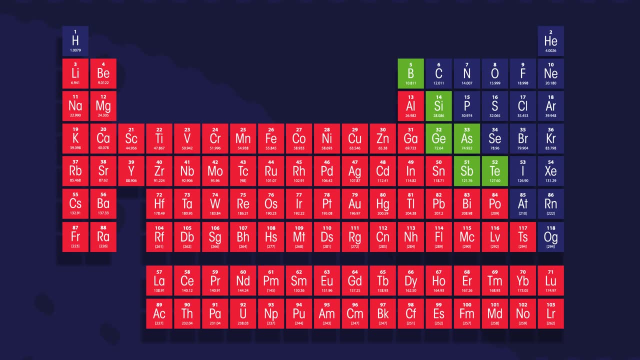 And now rewrite the list again. How did you do? From these two experiments we can rank all eight metals in order of chemical reactivity. This is, of course, a selective list, or else we would need to include over 70 metals. 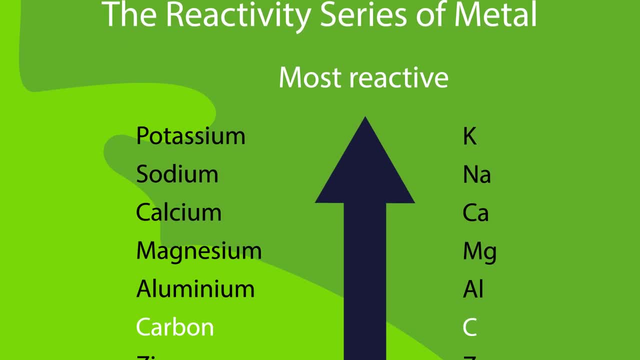 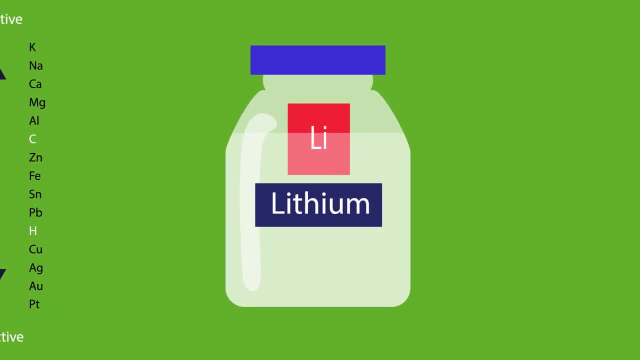 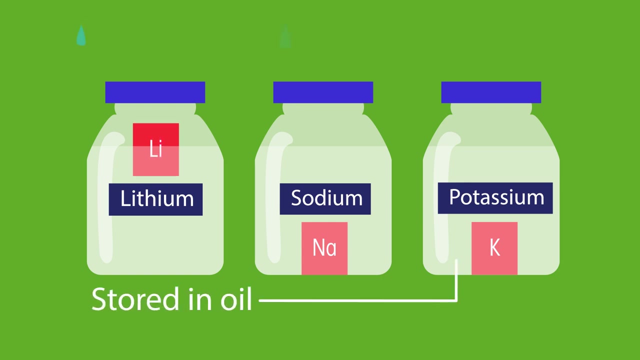 This gives us the reactivity series of metals, many versions of which you will find in books and online. You may already have known that Lithium, Sodium, Calcium, Magnesium and Sodium are the most reactive metals in the world. Sodium and Potassium were at the top of the list, since we store these metals in oil to 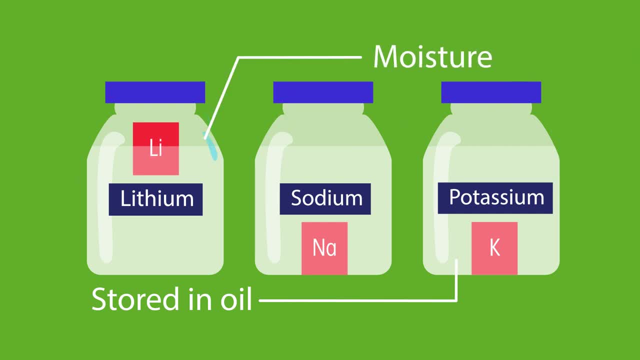 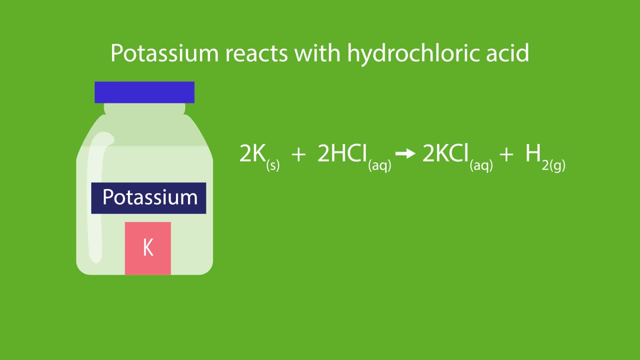 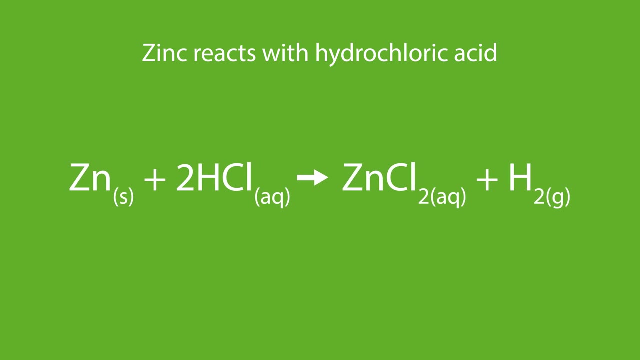 stop reaction with moisture in the air. When potassium reacts with hydrochloric acids, we get: Potassium readily loses an electron to form the K-positive ion, whereas when Zinc reacts, Zn will form its ion Zn2-positive, but less readily than potassium does. 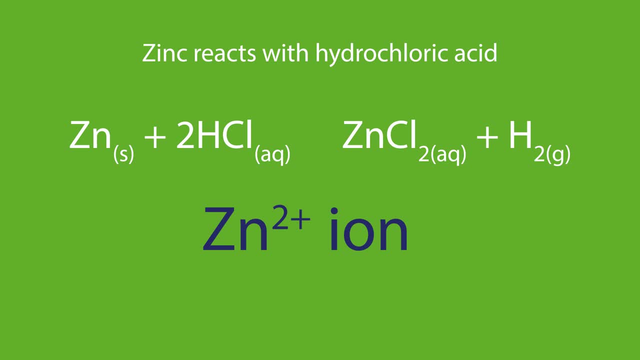 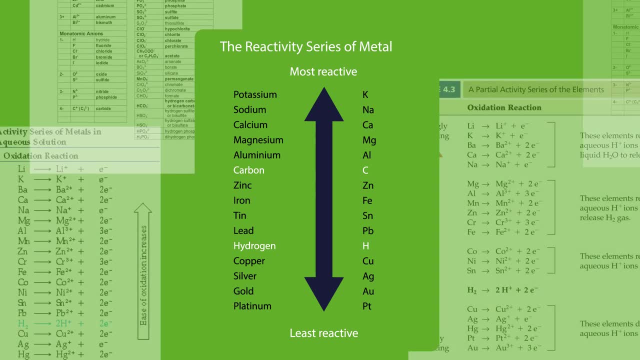 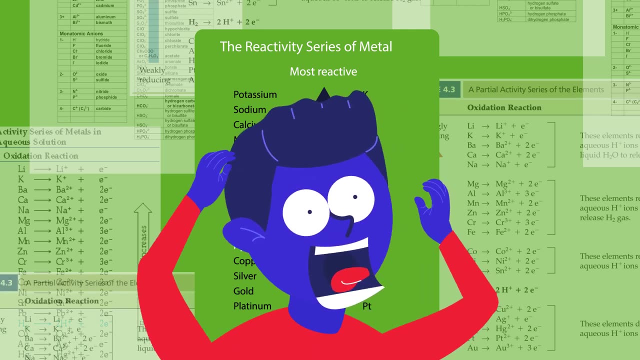 Potassium is the most reactive metal in the world. Potassium is the most reactive metal in the world, So the series of reactivity is also a list which shows the tendency for metals to produce their positive ions. Don't panic, you don't have to remember this list. 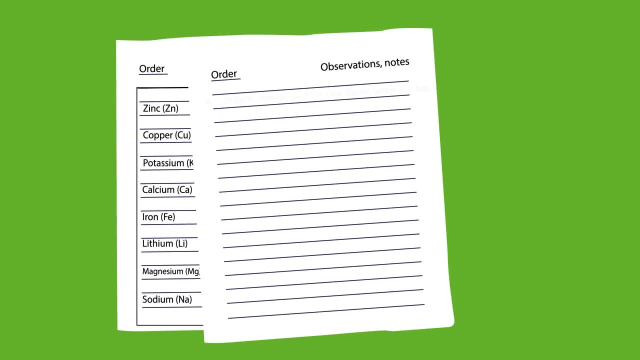 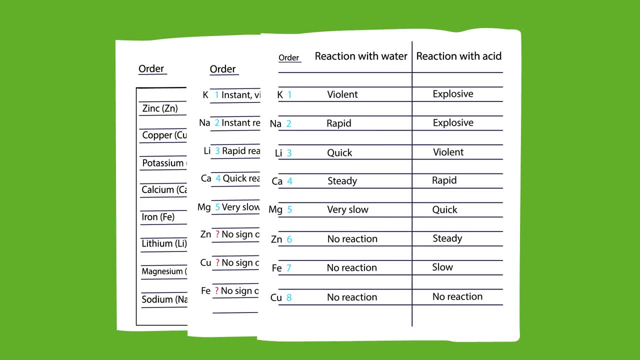 You should, however, be able to rank metals, if given results of an experiment, and then be able to use the list to answer further questions, such as in explaining displacement reactions. If you like the video, give it a thumbs up, and don't forget to subscribe and comment. 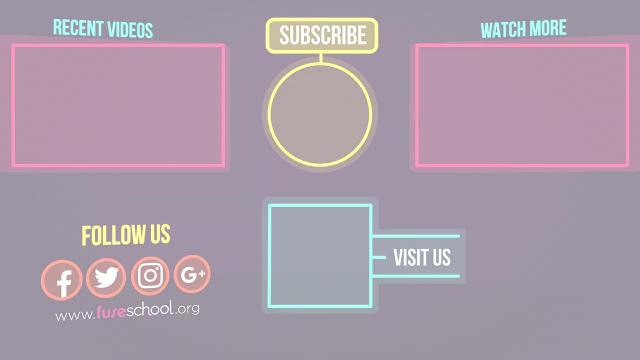 below if you have any questions. Thanks, H encompassing comparatively deepalin language. If you have any questions, why not check out our Fusco app as well? Until next time,